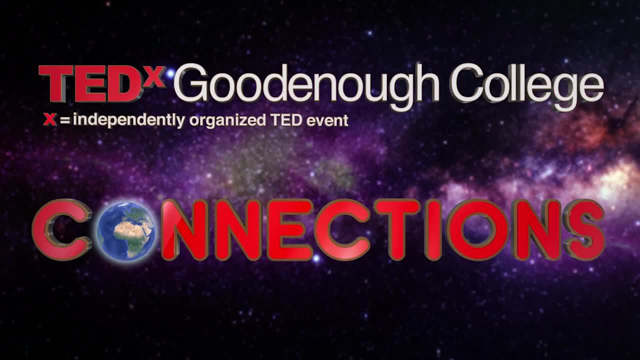 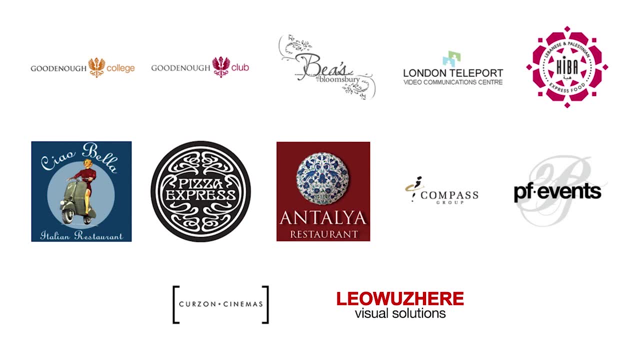 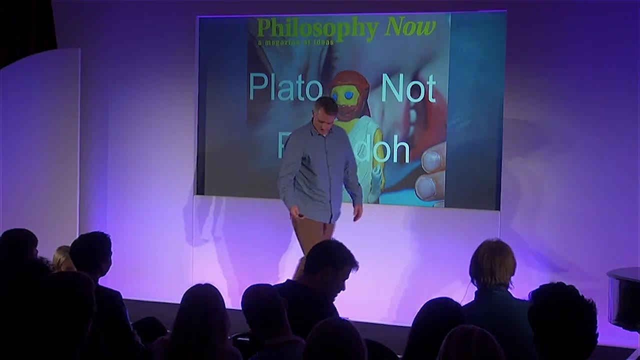 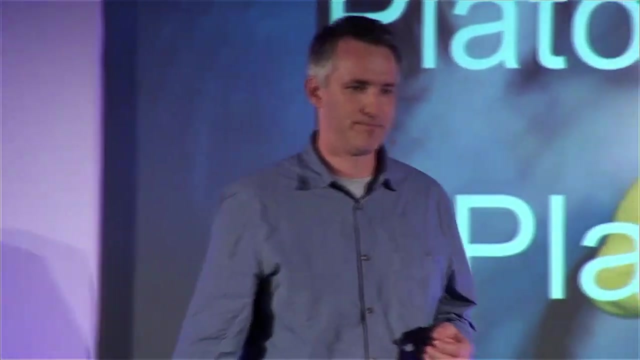 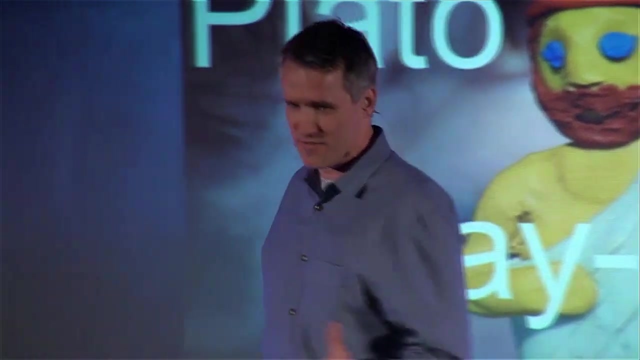 I'd like to begin by making the claim that philosophy is a kind of conversation. Now, I won't be the first to have made this claim. Two and a half thousand years ago, Socrates conducted all his philosophy in the form of conversations in the marketplace of Athens. 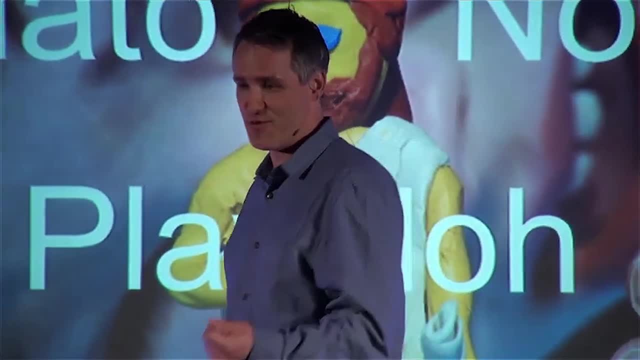 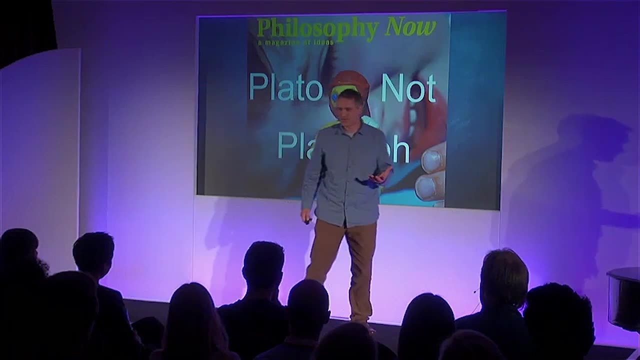 And present among the people. there was a pupil of his called Plato, And Plato wrote down many of these conversations in the form of dialogues that we still have with us to this day, And in one of those dialogues, the Phaedrus, 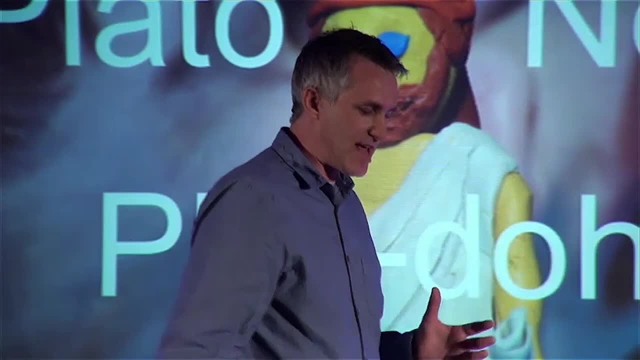 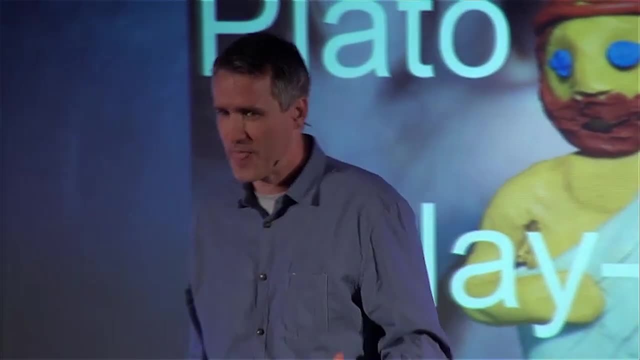 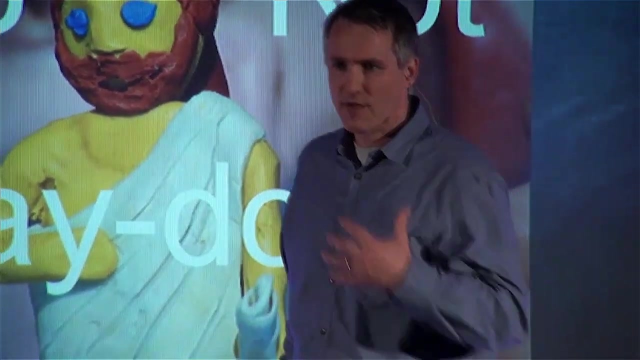 Plato has Socrates say that true philosophy can't be done through the written word. After all, books can't answer back, They can't qualify or clarify or respond. reply to objections: No, for Socrates, true philosophy can only be done. 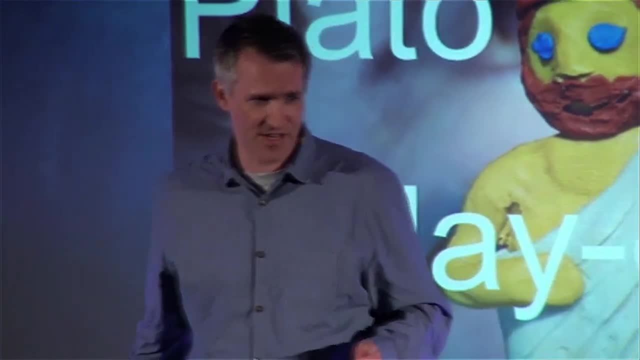 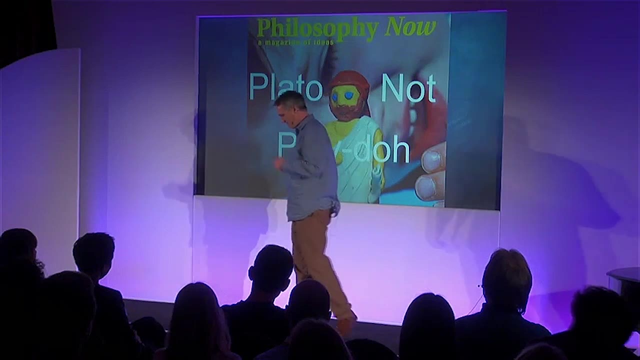 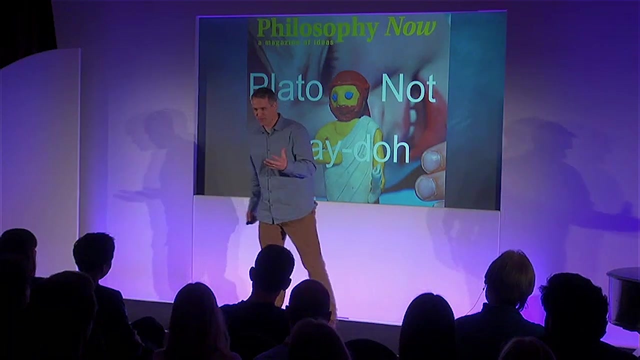 through a living, breathing conversation, As Lewis Carroll would have Alice say many years later: what's the use of a book with no pictures or conversations? Now, there's an art to conversation, And one is most acutely aware of this when one is engaged in talking. 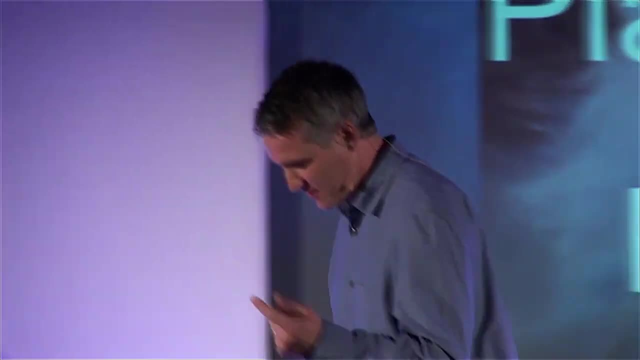 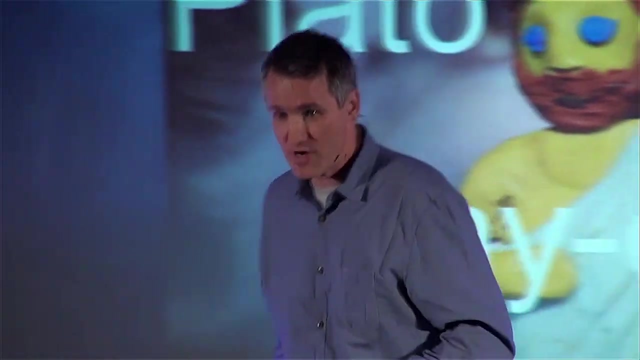 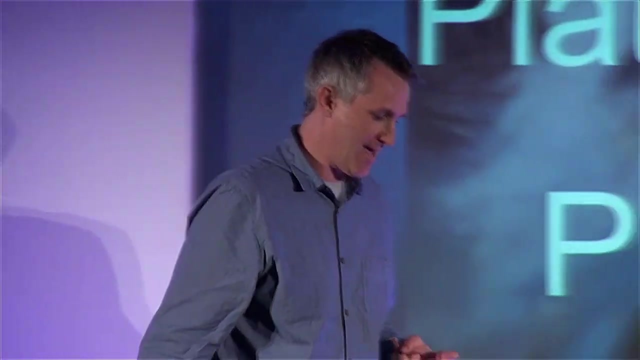 with someone who has no sense of it. For instance, some of you may be familiar with talking with someone who constantly monologues, who asks no questions, or at least only rhetorical ones, and who doesn't listen to the other speaker. Yeah, a little bit like me today. 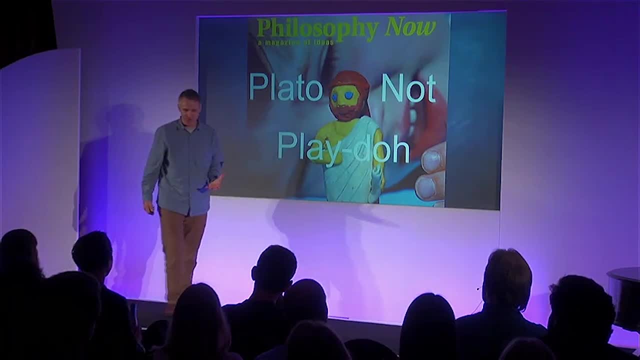 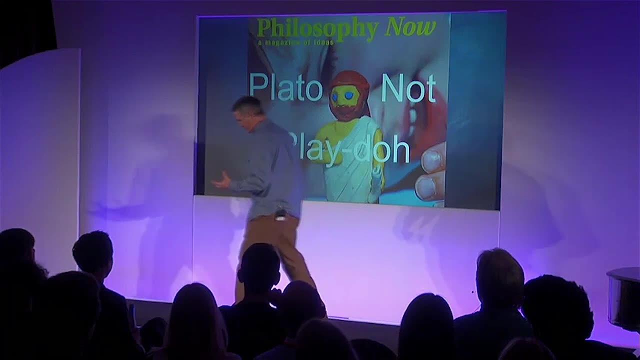 See, I find myself in a slightly awkward position here, standing before you Extolling the virtues of conversation whilst not actually engaging in one. So I will ask you to bear with me, But, in order to get around this, what I may do from time to time, 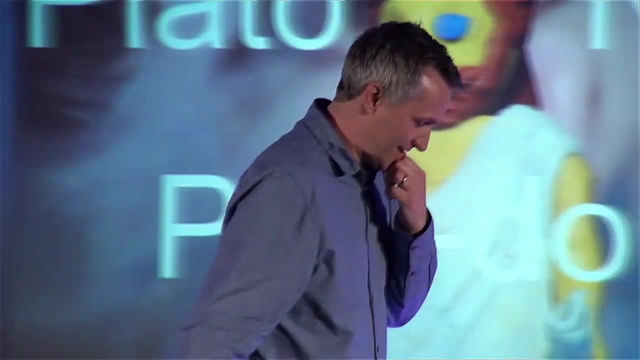 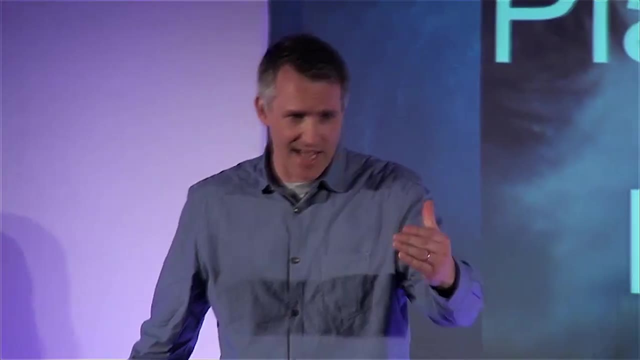 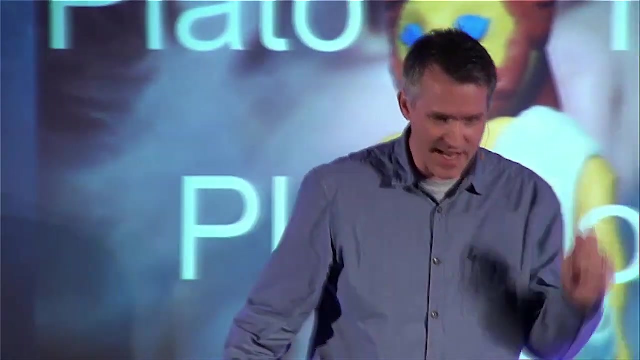 is have a pretend conversation with you. Now, where was I? I need that on-stage prompt. Ah yes, conversation is a kind of two-way thing. It has an interactive back and forth and it's like tennis. But what's essential to that interactivity is that it be meaningful. 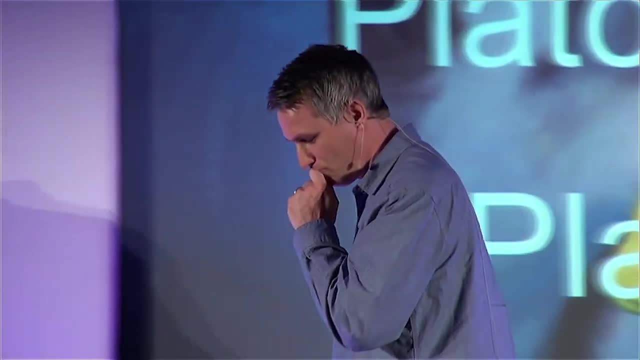 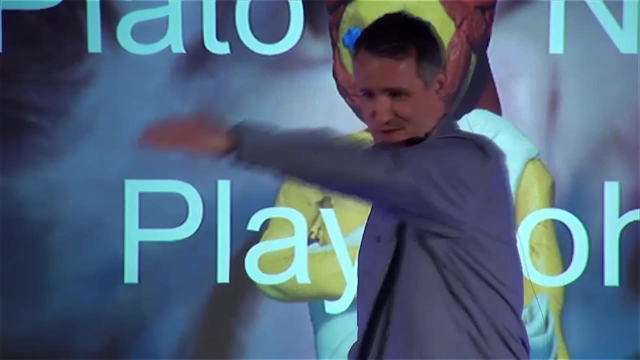 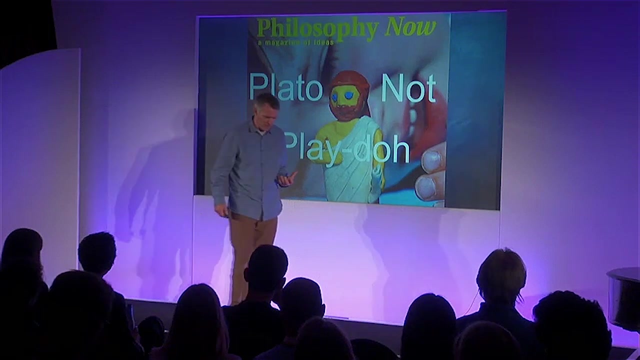 meaningfully connected. I do philosophy with children. I go into schools and I set the classroom up in a big circle. I ask the children to, I ask them questions, I give them puzzles, stories, all of a philosophical nature. For instance, I might ask them the famous Harris-Clytus question. 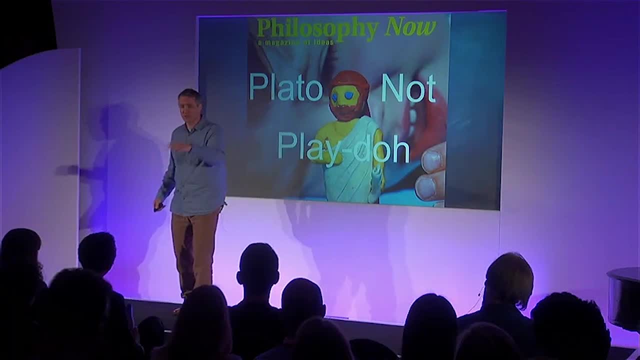 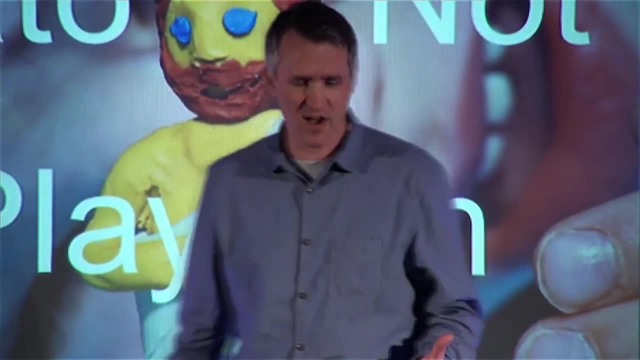 can you step in the same river twice? Then I facilitate a discussion amongst the children ages 3 all the way up to 19 and above, And one of the questions I often get asked when I tell people what it is I do is: but can children do philosophy? 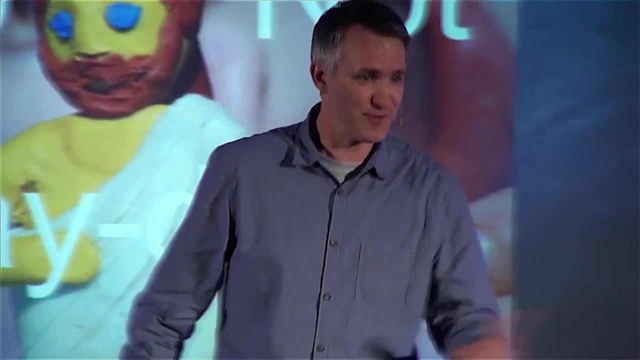 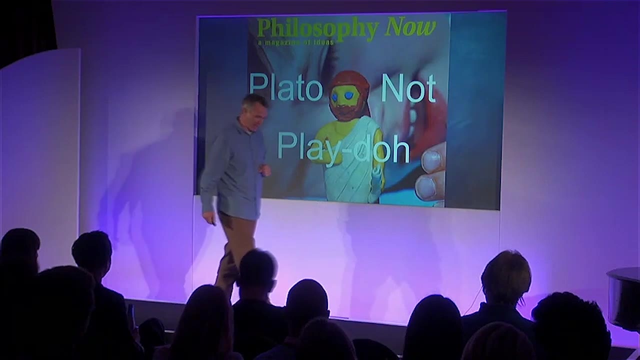 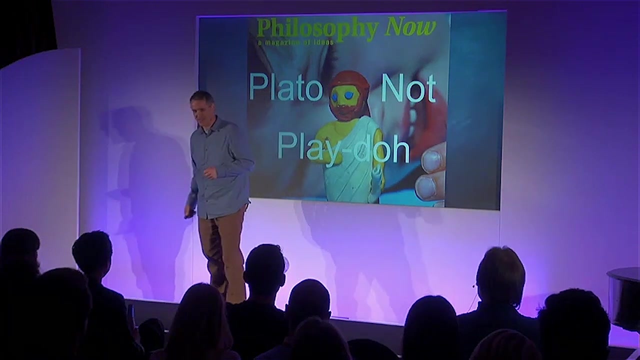 So I'm going to have you ask me that question now. Can children do philosophy? Yes, Well, that was easy. Well, one of the standard replies that people give to that question is, of course, yes. practitioners of philosophy with children will say that. 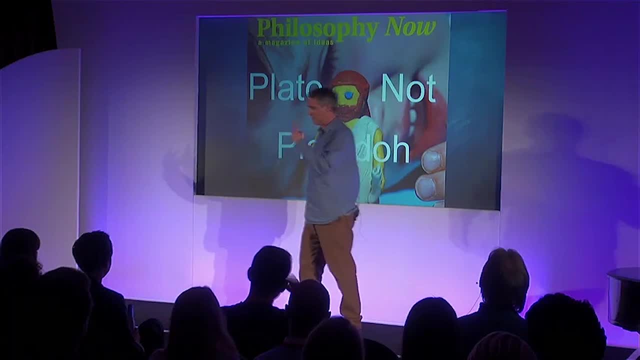 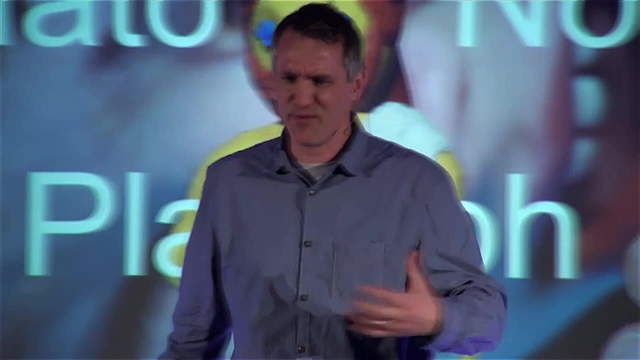 And they'll say things like: well, we give them genuine philosophical questions, they have plenty to say about it, they engage with the questions and they really enjoy doing it. But then I hear you say: but can they really do philosophy? 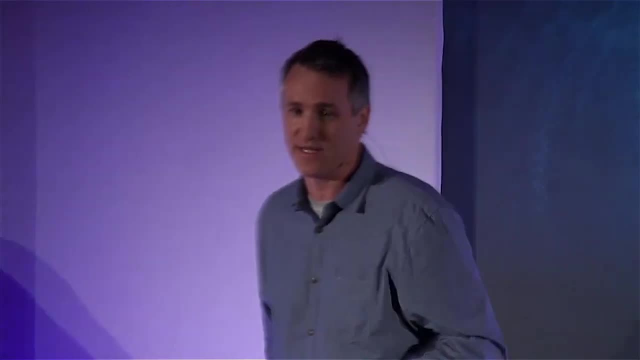 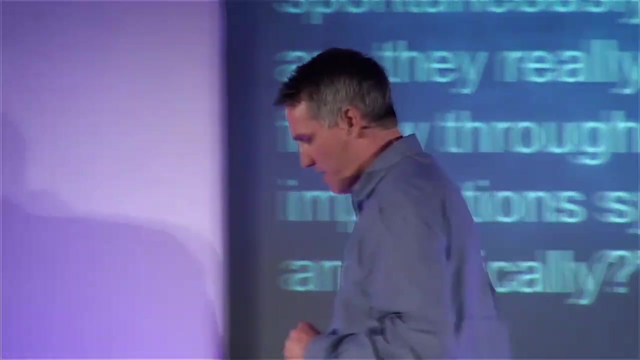 That's not very well, but can they really do philosophy Now? if you're one of those who still remain sceptical after my powerful argument, then you're not alone. Julian Beggini, philosopher. Julian Beggini said that children can really astonish with the spontaneous philosophical ideas that they have. 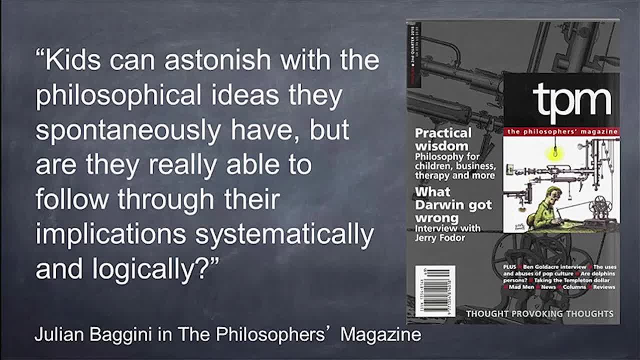 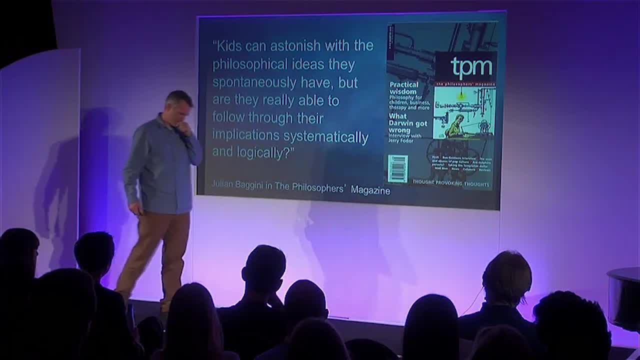 But he asked: can they really follow through the implications? Can they really change their ideas systematically and logically? And isn't that what philosophy is about, Not just having interesting ideas? Well, earlier on I said that philosophy is a kind of conversation. 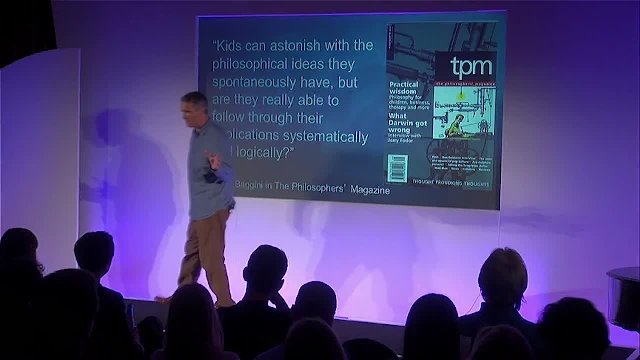 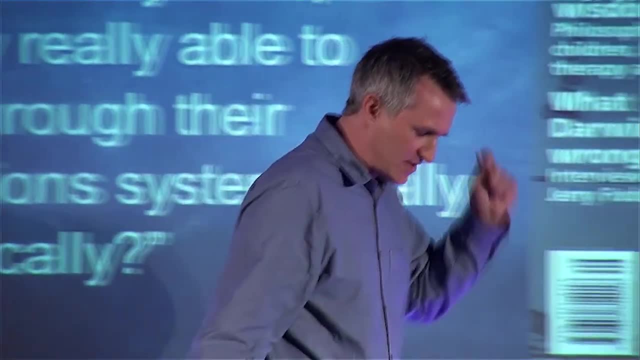 I should point out, it doesn't work the other way, though. Not all conversations are philosophy. One can have a conversation about what you're going to have for tea tonight, for instance, So what is it that's special about a philosophical conversation? 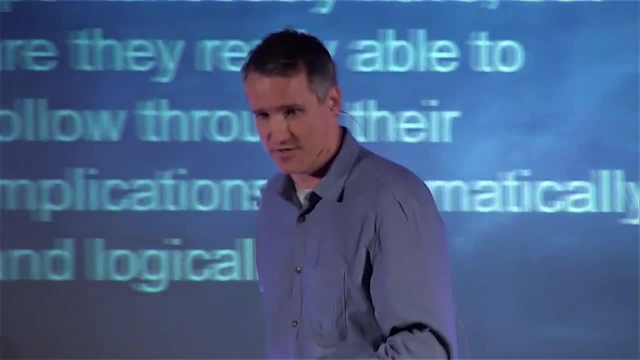 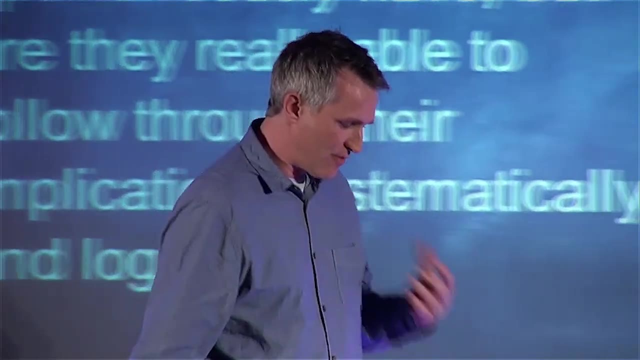 I would say it's to do with the responses and the connections And I want to say something about and I want to say something about that by saying something about what philosophy is. So I'm going to run through three conceptions: common conceptions of what philosophy are or possibly misconceptions. 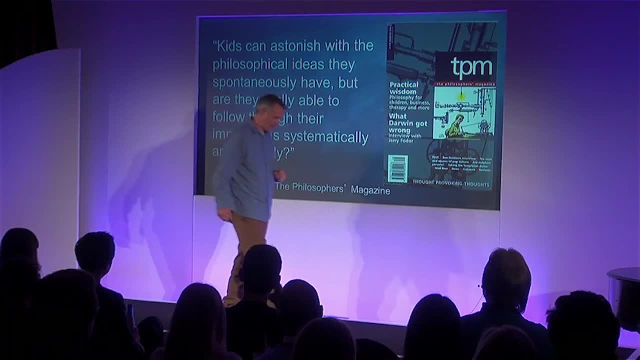 And then I'm going to appeal to the children to clear them up for us. So one of the conceptions is that philosophy is about asking questions, which of course to some extent it is, But I much prefer nine-year-old Oluwaiode's idea when she said: 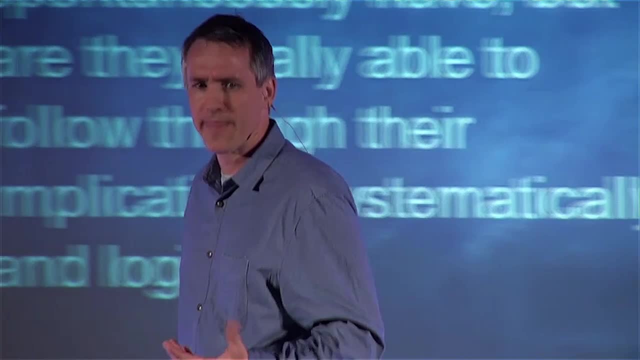 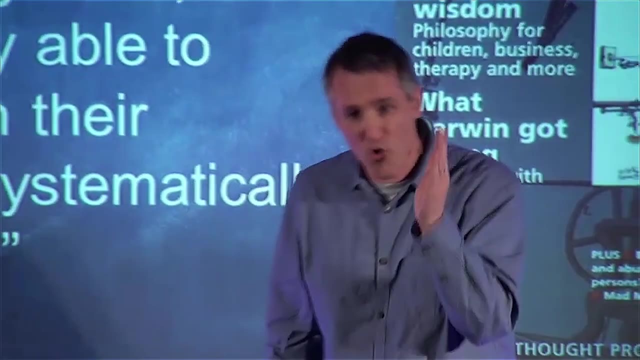 isn't philosophy really about understanding questions? So this is much closer to the mark for me. Philosophers do ask lots of questions, but they spend an awful lot of time on the question saying: is this the right question? Has this been asked in the right way? 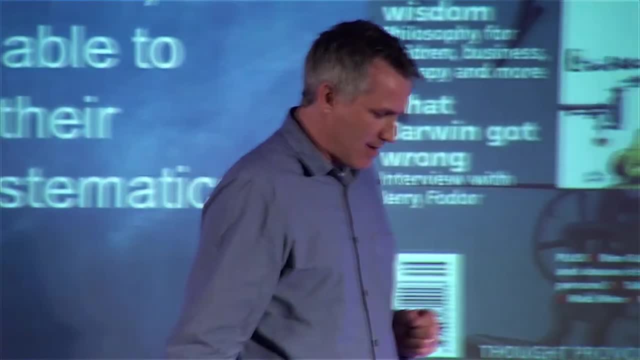 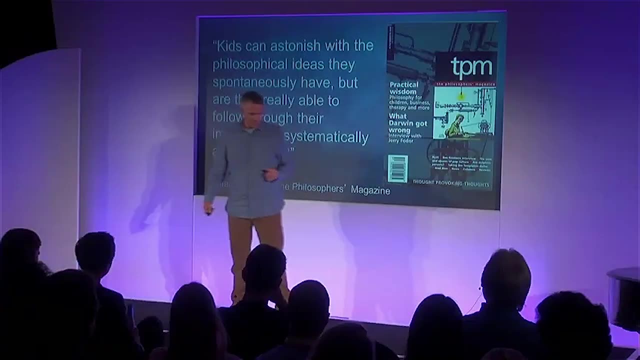 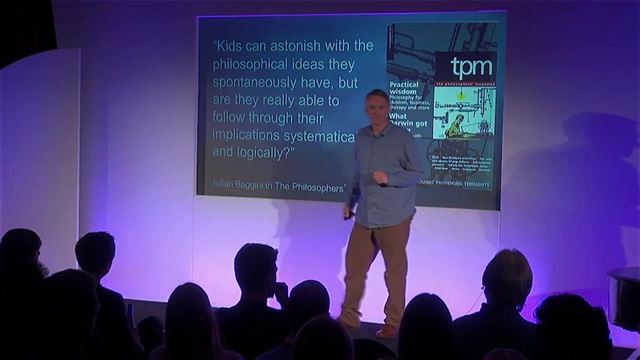 Is there a better question? Another conception is that philosophy is about answering questions, And for many people the big question is no less. Well, this often leads to disappointment, I'm afraid to say. I much prefer ten-year-old Amy's response. 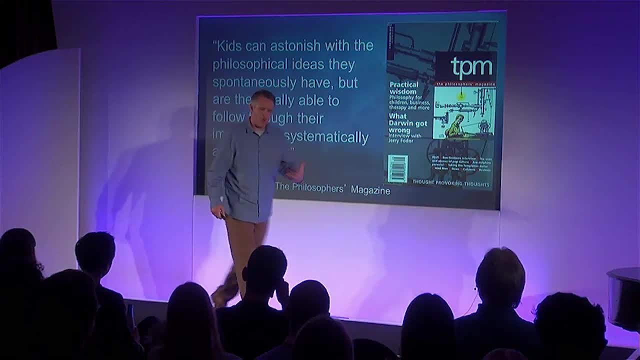 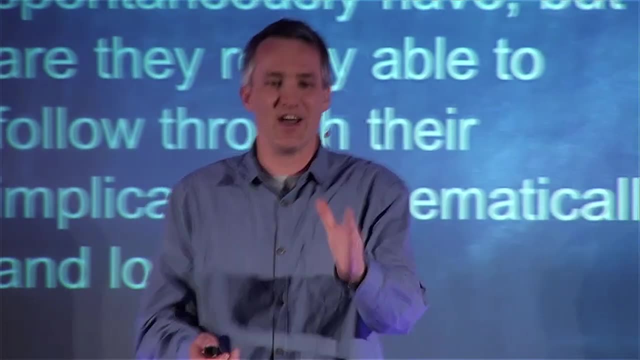 when she said that philosophy is about, isn't it about? exploring possible answers? And this again seems much closer to the mark. What philosophers do is they take the candidate answers that there are and they look at them and they explore which ones they could pursue. 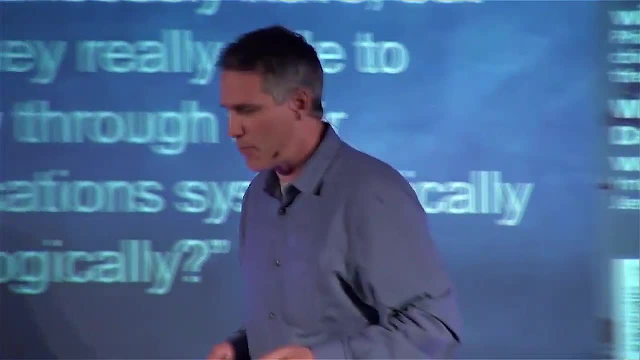 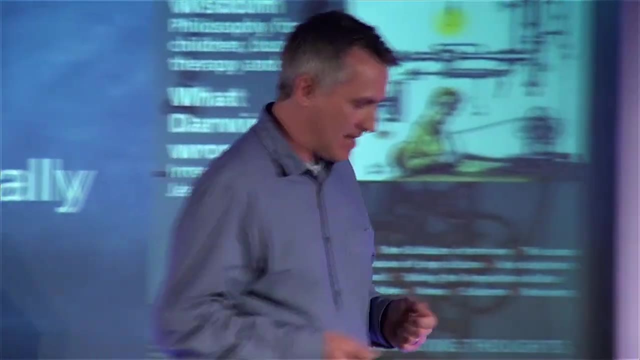 And in some cases then pass those questions over to the sciences to perhaps try to answer them. What philosophers do is they kind of pave the way. And then finally, a lot of people think. People think that in philosophy there are no right and wrong answers. 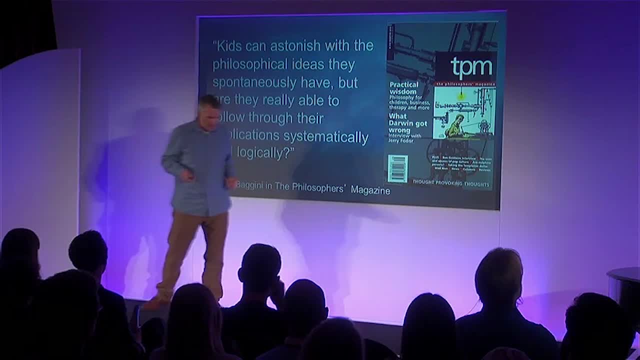 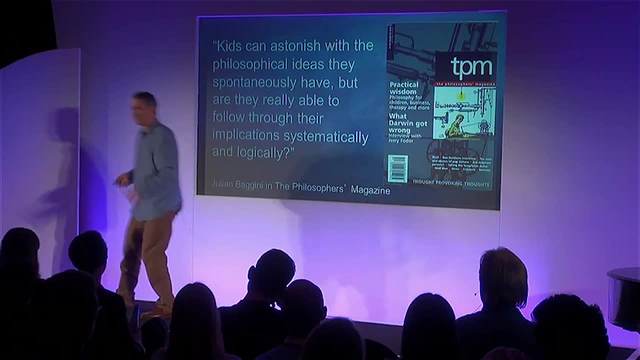 But, said 11-year-old Adam, what's the point of philosophy then if there are no right and wrong answers? He said there are right and wrong answers in philosophy. it's just incredibly difficult to know what they are. This, I think he hits the nail on the head. 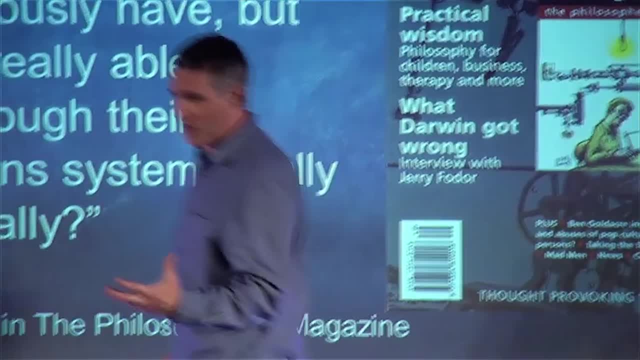 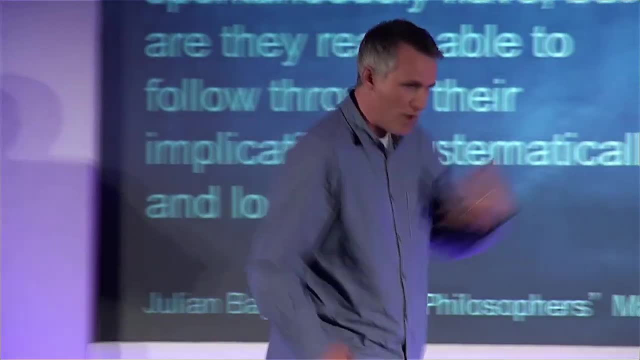 Now philosophy also begins well. Plato said it begins in wonder. I'd be more inclined to say that philosophy begins with puzzlement. You see, most of us at some point bump up against the world. We find the world strange, odd, puzzling, sometimes contradictory. 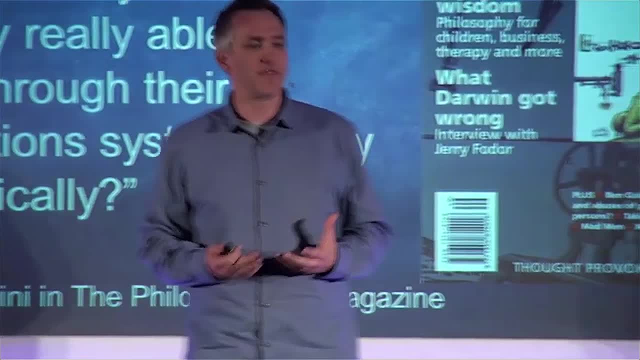 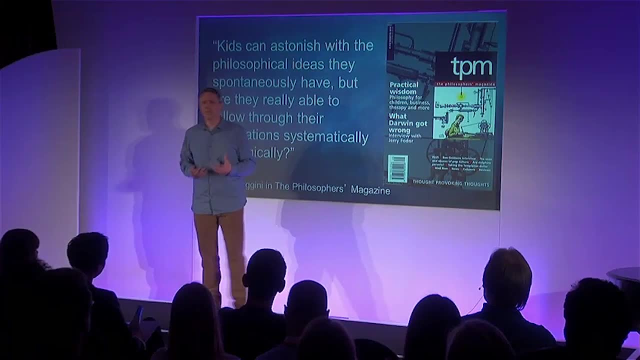 To give one example, a child in a classroom might think that fairness is when you share things equally or you're treated equally. But then they see another child in the class, perhaps a child with special needs of some kind, who's getting more attention than the rest of the class. 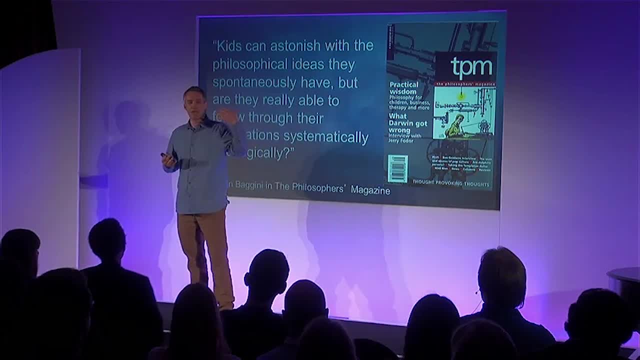 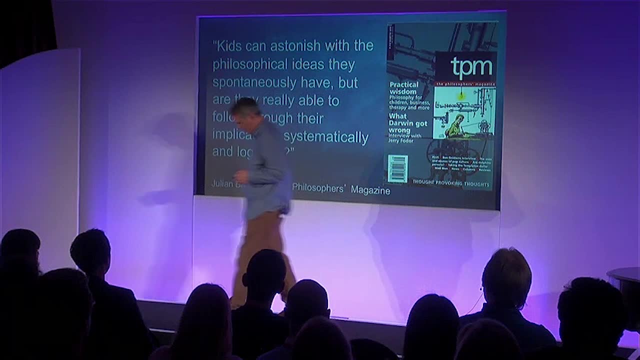 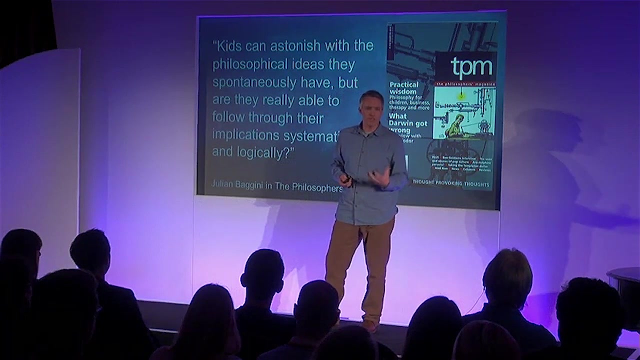 And maybe that child doesn't yet have a concept of fairness, as fairness in the classroom And that's according to need, So it doesn't quite fit The world's not fitting with how they see things. Well, I would say that philosophy is about the responses that we have. 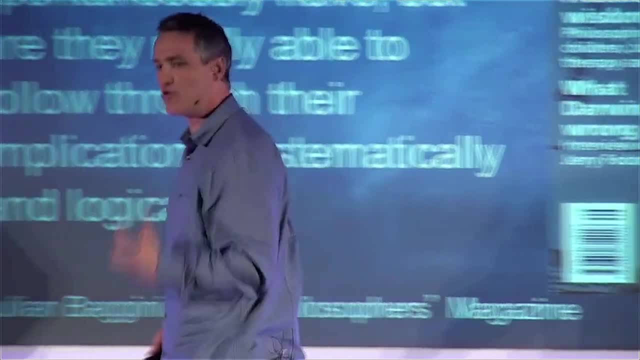 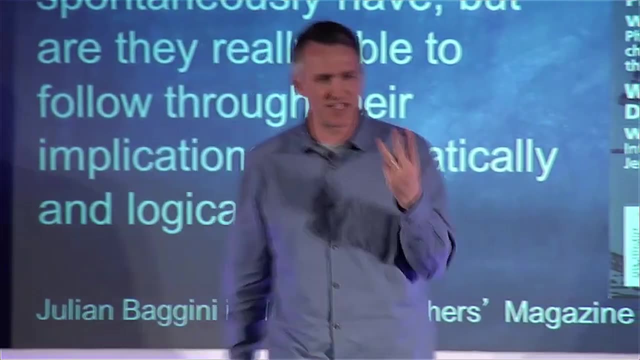 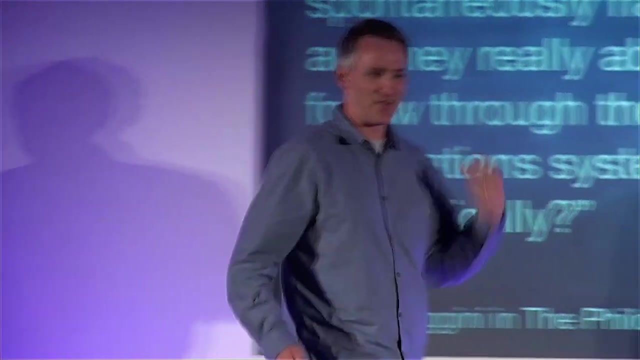 to those kinds of experiences, And it's the special kind of responses that philosophy has that I want to draw your attention to. So I'm going to make the claim that there are three central ideas, each beginning with the letter R. This is the three R's of philosophy. 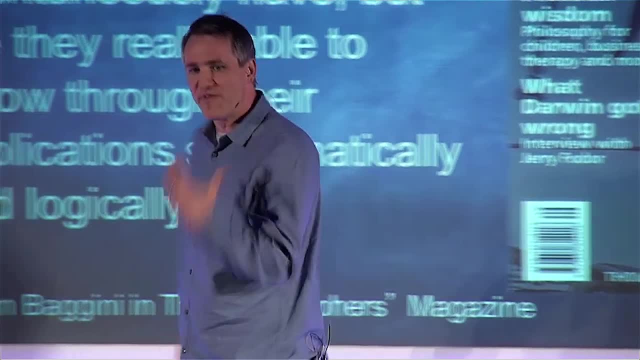 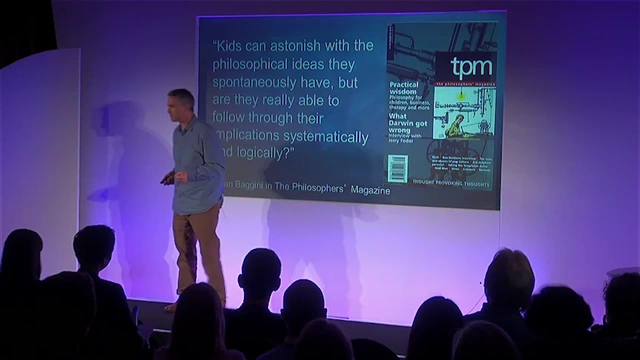 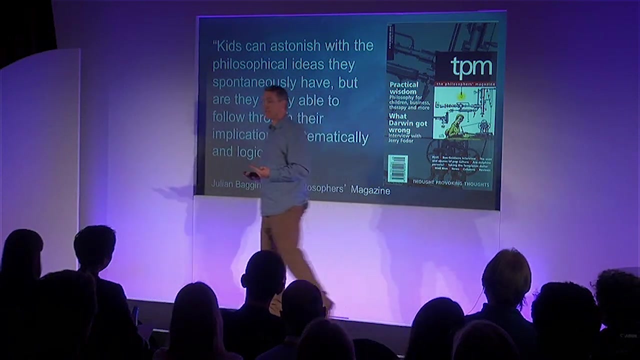 The first is that when we respond philosophically, we do so reflectively. We stop and say: what is X? Or, in the case of the child, what is fairness? Secondly, we then try to answer that question by a method, a systematic method of reasoning. 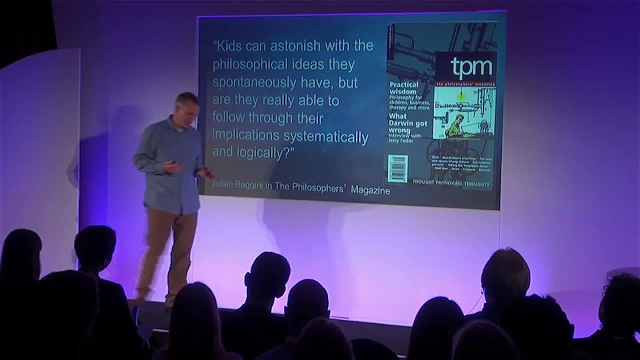 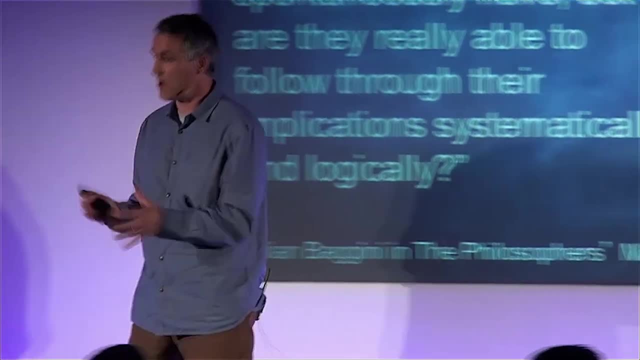 And then, when we've done that, we don't stop there, or philosophers don't stop there, because the third response has to be: is this right? It has to be re-evaluative: Is this the right answer? It needs to be subjected to some sort of critical analysis. 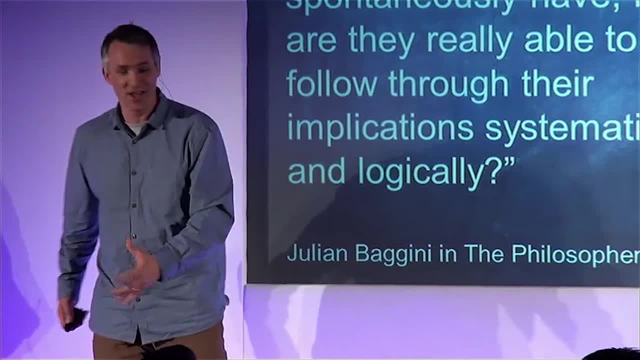 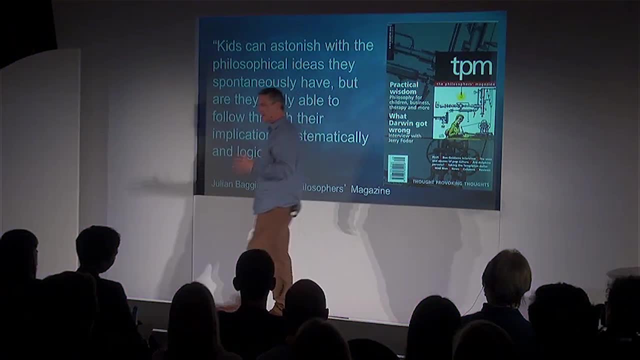 Now I could talk a long time about how children can do these things, but I would much rather show you. So I'm going to show a short film and I'm going to introduce you to 11-year-old Noah and 8-year-old Alice. 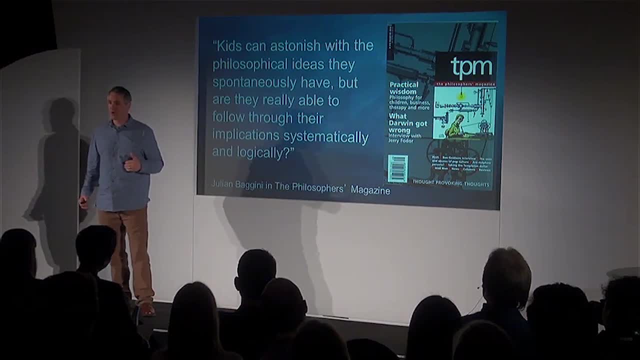 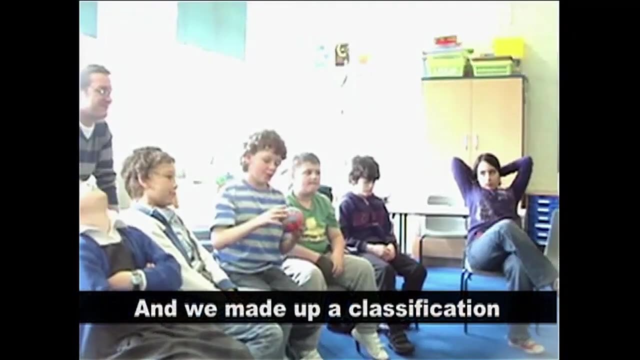 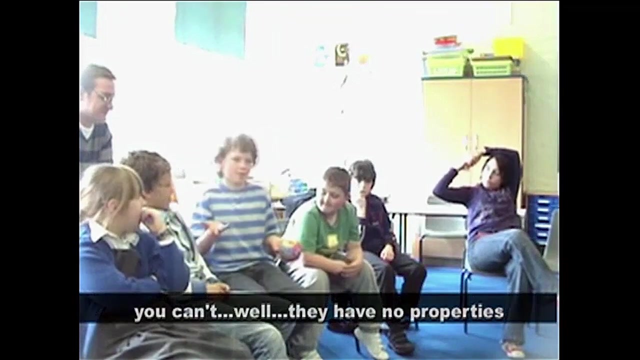 But I really want to draw your attention to Alice at the front with the blue cardigan on Watch her arm. Now we need a classification for things that have no touch. smell you can't. well, no properties, but do have consequences. 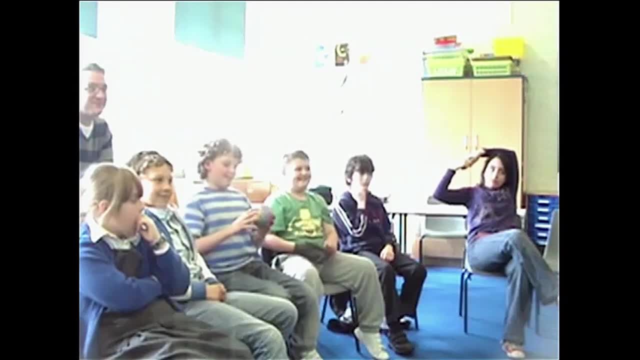 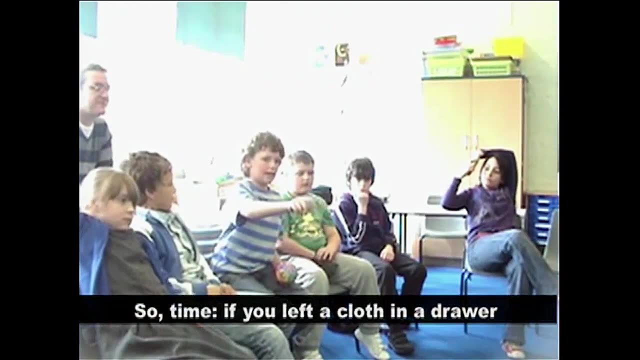 We call them anti-things. So things that don't have properties are called anti-things, But they do have a consequence. So time, if you left a cloth in a drawer, it would get dusty. That is a consequence of time. 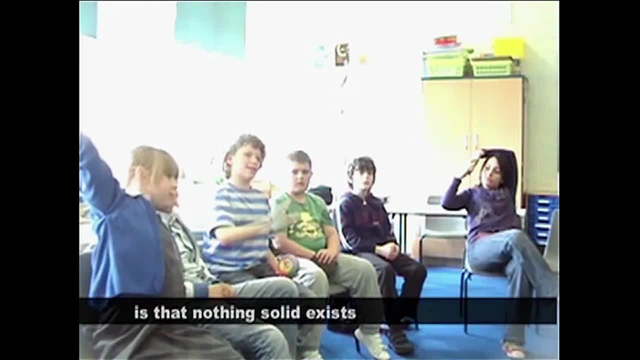 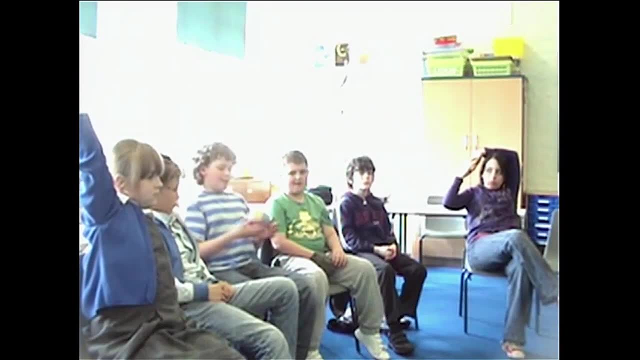 Nothing. the consequence of nothing is that nothing solid exists. The consequence of existence is the exact opposite. Solids appear, Some, that would some, and also all forces they have. they have you can't. they have no properties. 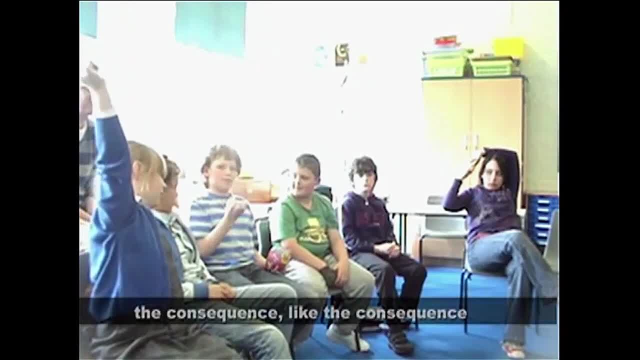 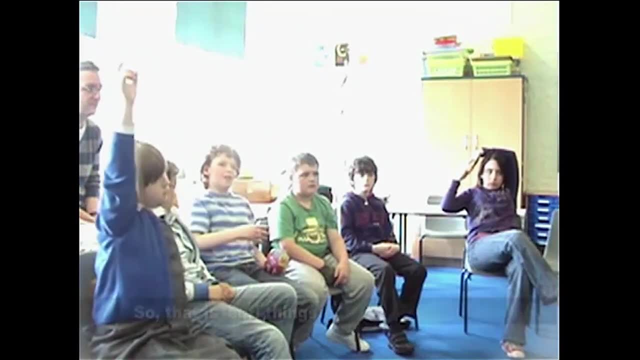 but the consequence of vanity is that you can go down if you go up. The consequence of motion is that if you're going downhill you'll speed up. So that is anti-things. no properties, but they do have consequences, Wow. 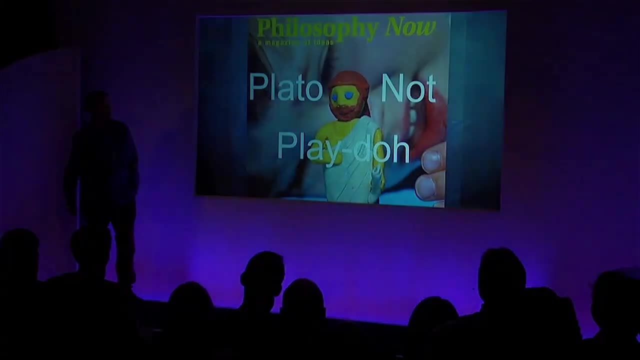 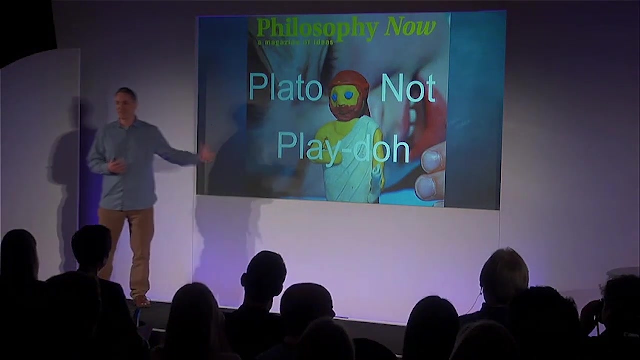 That's the best laugh, biggest laugh I'm going to get. So many of you, I'm sure, will share in Rokas' wow at Noah's big idea. And it really is, you know, and yes, we should. 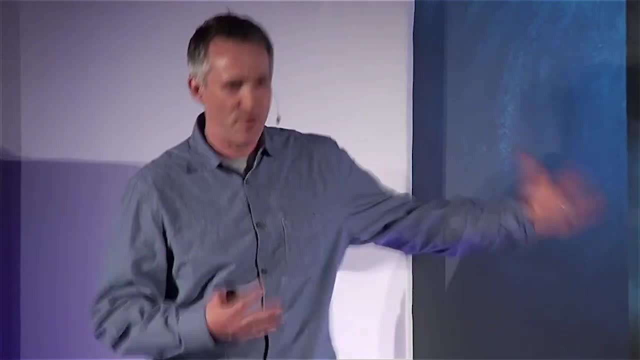 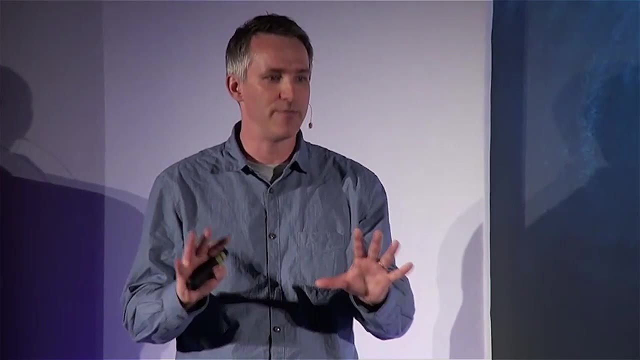 I mean, a lot of practitioners of philosophy with children will probably leap on this example as an opportunity to show you children doing real philosophy. But I'm going to ask you to be calm here. Don't get too excited, Because yes, there are lots of features of philosophy there. 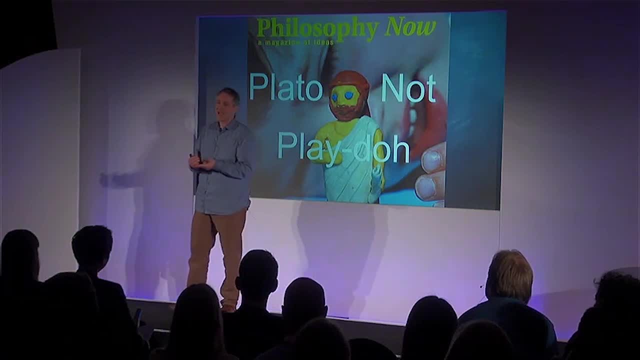 He's constructing a complex argument, He's thinking abstractly, and he's doing so about general things. He's thinking about metaphysics, in other words, the nature of reality, and he's doing so conceptually, which is so central to philosophical practice. 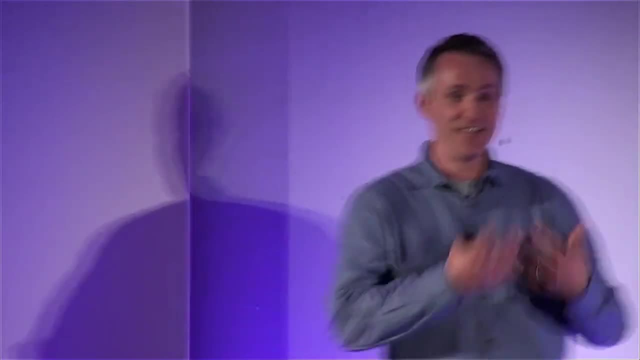 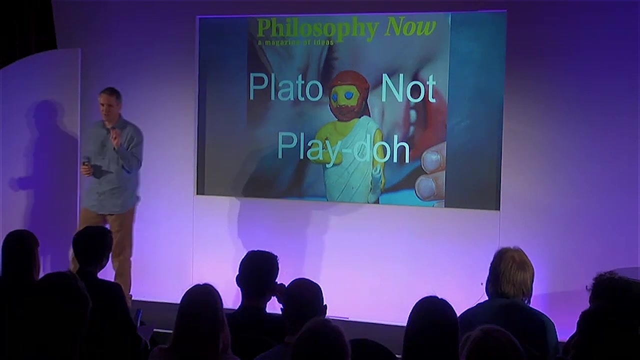 He's even had an original idea and he's come up with his own word: anti-things. This is what philosophers do, almost. There's something missing at this stage to call it good philosophy- that we find with Alice's response. 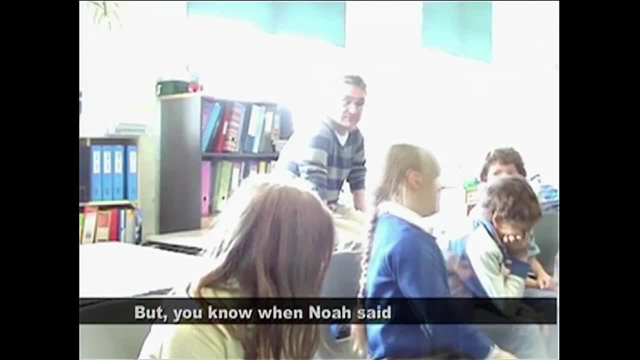 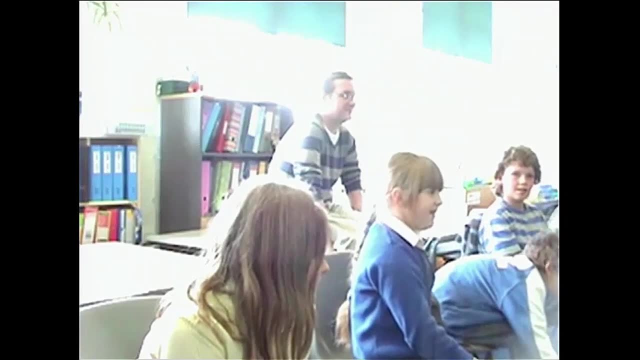 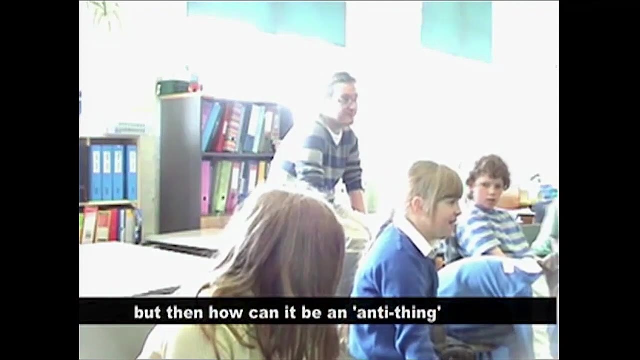 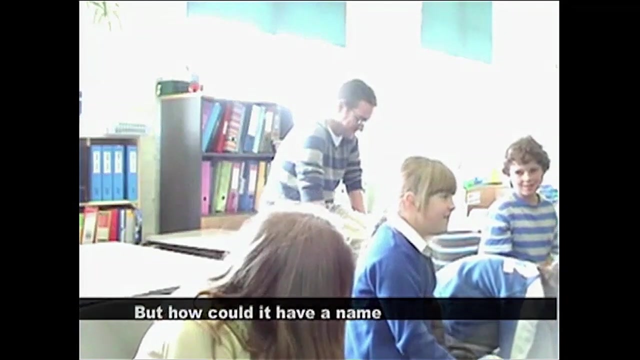 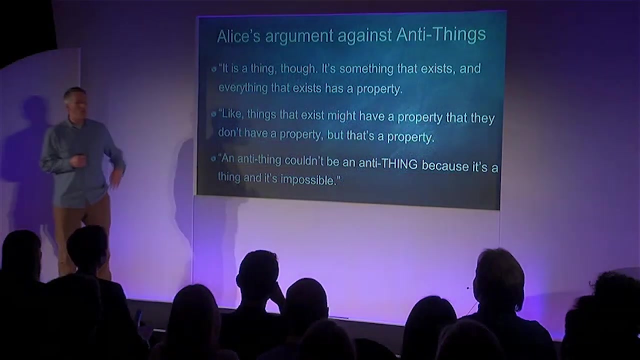 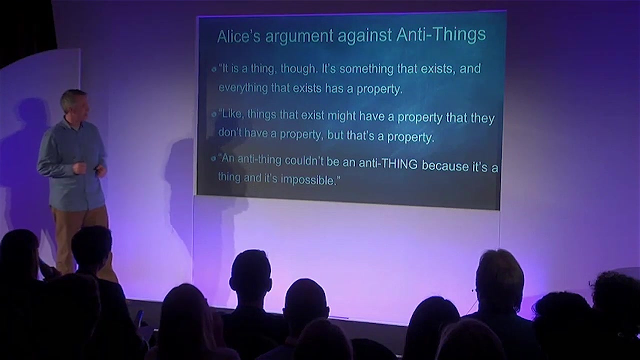 And, of course, a week later, she came back, having thought about this, and she said this: It's a thing, though it's something that exists, and everything that exists has a property, Like things that exist might have a property. 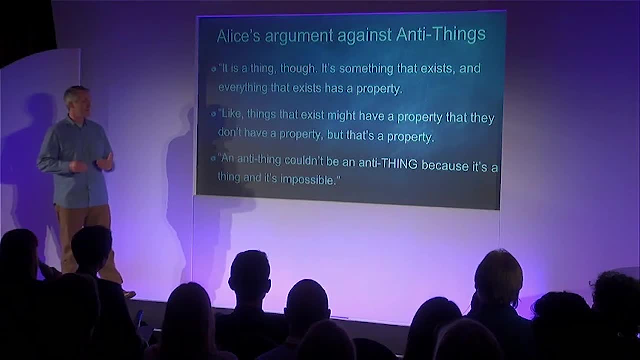 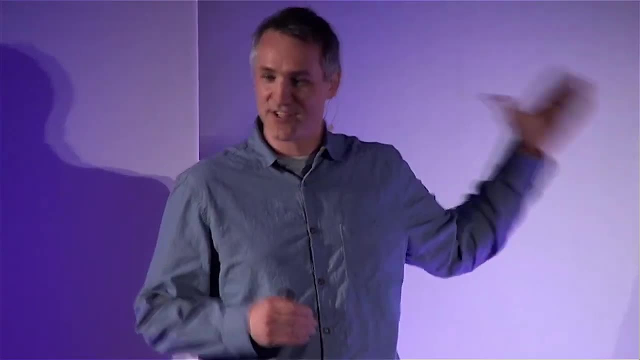 that they don't have a property. But that's a property. An anti-thing couldn't be an anti-thing, because it's a thing and it's impossible. Alice is asking all the right questions. She's now inviting that extra element that I talked about. 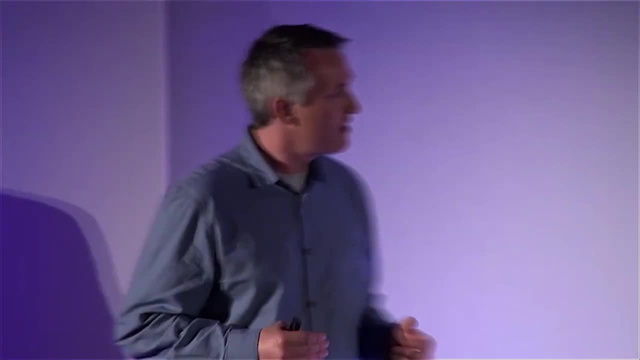 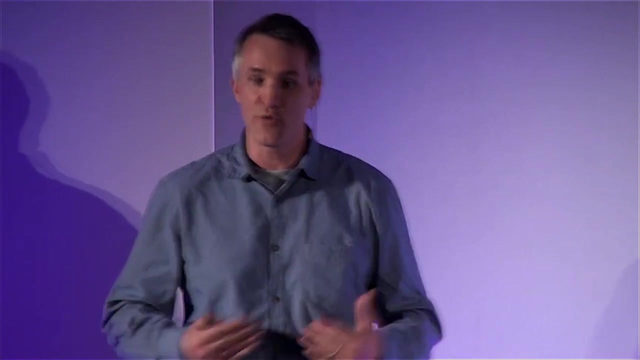 the re-evaluation. She's being critical, But she's not just being critical in a negative way or randomly. She's doing so according to the logical demands of what it was that Noah said: Let's have a look. So, for instance, she's come up with a principle, identified a principle. 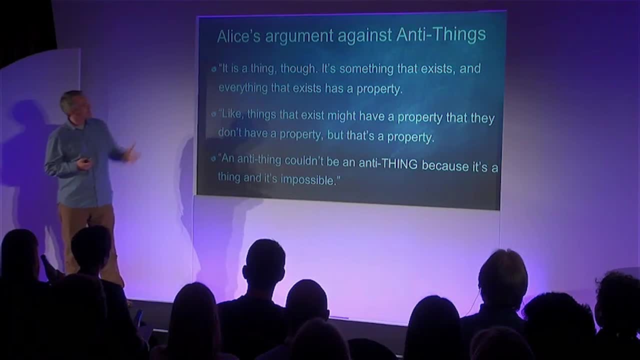 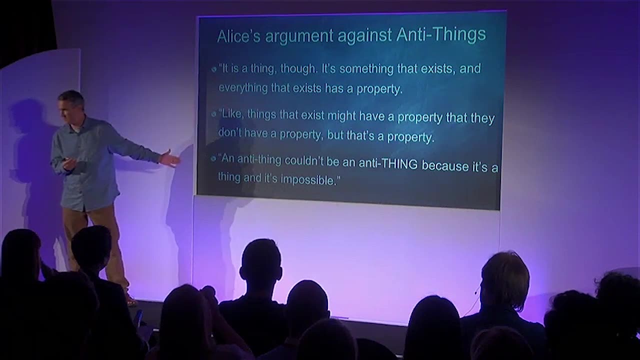 Maybe we can call this Alice's principle, that existing things necessitate at least one property. you could say She's also noticed that it might have a self-refuting quality to it. So the property of having no properties, itself being a property, might be self-refuting. 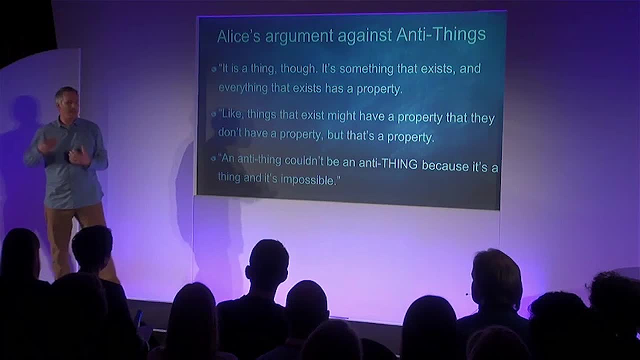 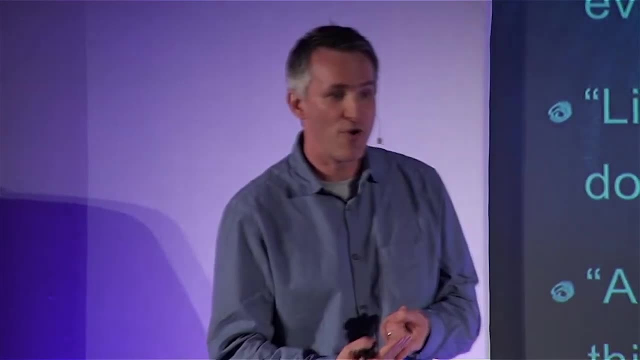 So she is now challenging Noah. He has to re-evaluate his theory, his great theory, And he's going to either have to go away and revise it or he's going to have to reject it. This is the key thing. 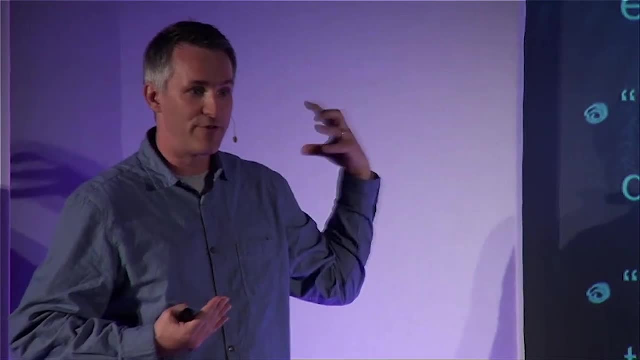 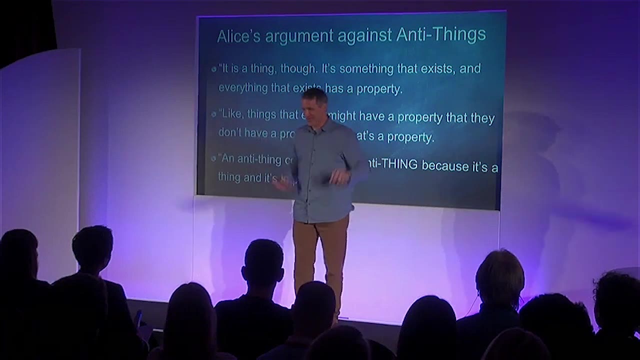 So when we see Alice's response in conjunction with Noah's big idea at the beginning, we see some good philosophy. So in answer to the question that you asked me at the beginning: can children really do philosophy? Yes, they can. 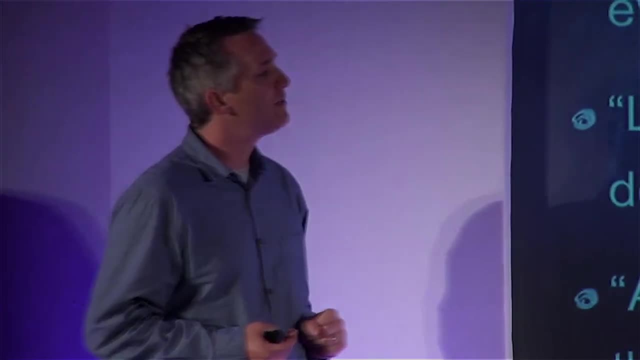 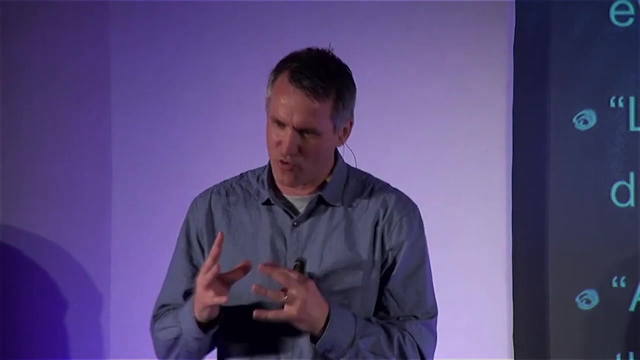 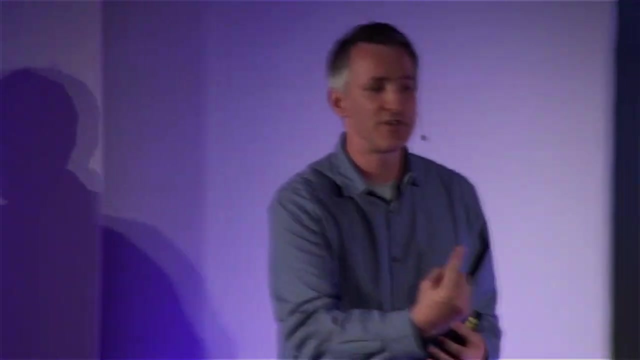 But I would offer a qualification. I think children can do philosophy, but they tend to struggle with it when they're on their own or if there's just two of them, because they lack the variety of responses that are necessary to sustain a philosophical conversation. 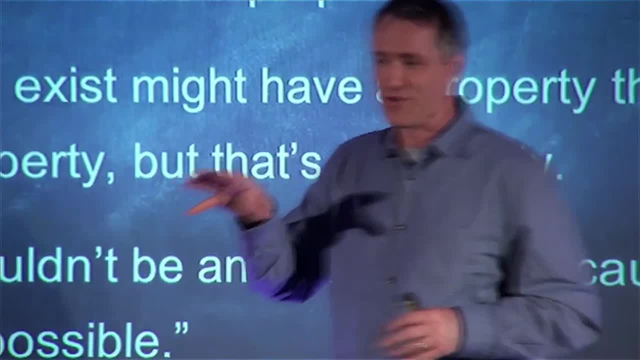 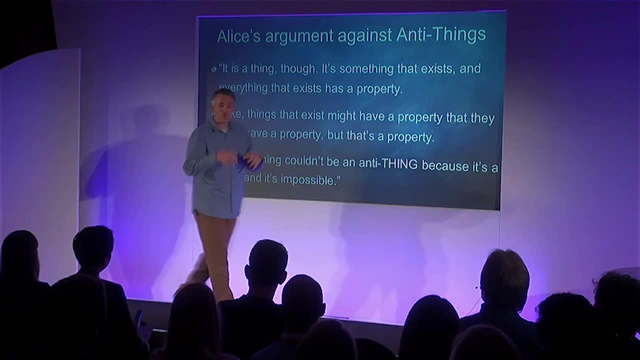 However, if you take 20 children or 30 children, put them together, then they start to have the variety of responses that are needed And with a little bit of facilitation they can also have the right kinds of responses, as you've seen tonight. 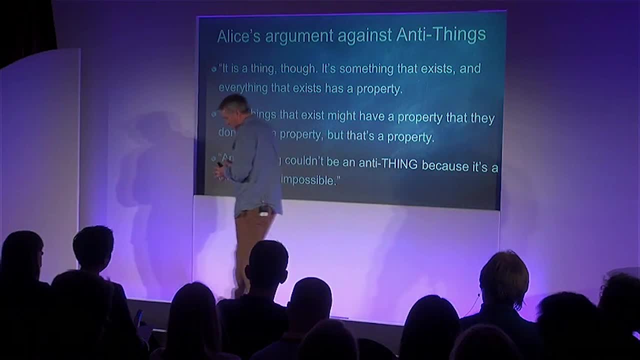 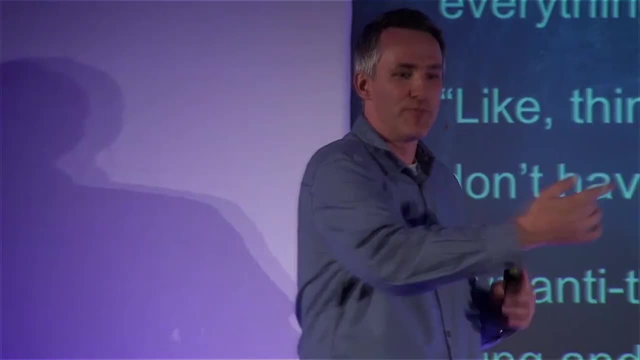 in order to be able to have a philosophical conversation, And at the Philosophy Foundation, the thing that we very much aim to try and do is to have the children watch each other as they do the philosophy, and then they start to learn how to do philosophy on their own. 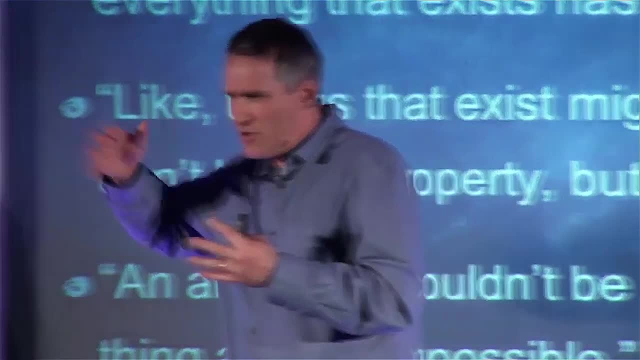 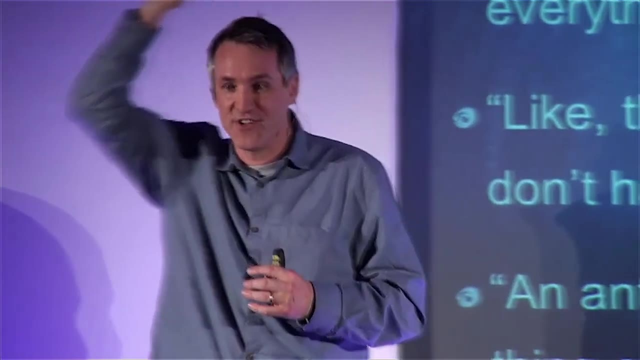 by watching them do it as a class, And they start to see how to interact with each other, but also with themselves, And then they start to learn to have what Socrates called the silent dialogue, this dialogue, This conversation that we have in our own heads when we think things through. 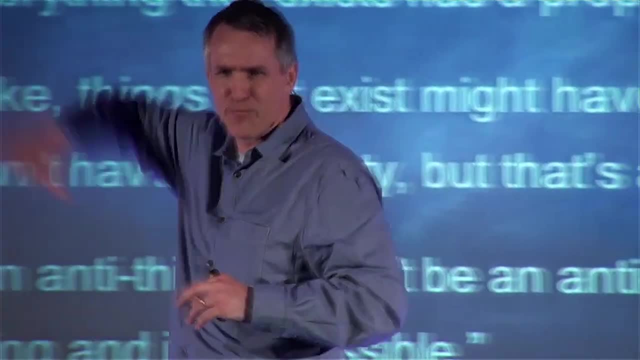 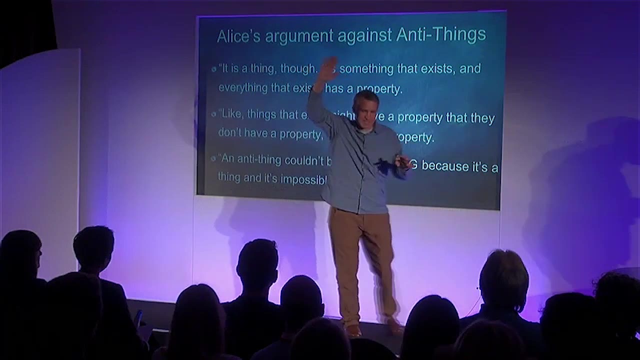 And we know this sort of thing's going on. when children say things like Miss, because I'm always Miss, by the way, Miss, I'm going to say something which disagrees with myself now. So when the children start to say those sorts of things,